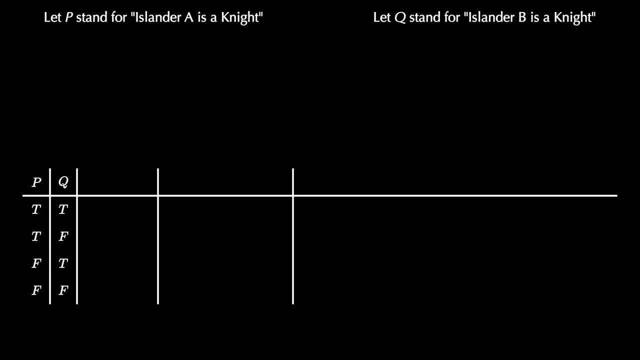 And the truth table has a column for P and a column for Q and four rows for the four possible truth situations. Person A says: if B is a knave, then I am a knight. This is a truth table. This can be interpreted as not: Q implies P. 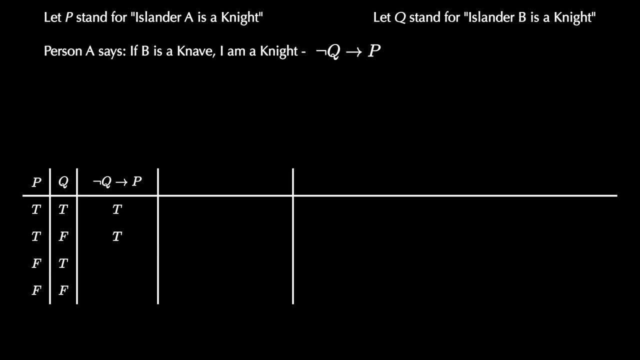 Because this is a connective between two atomic propositions and is a conditional. there's exactly one place where it's false, and that's in the bottom row. Person B says something more complicated. A could claim that I am a knave. We can interpret this as P and not Q, or not P and Q. 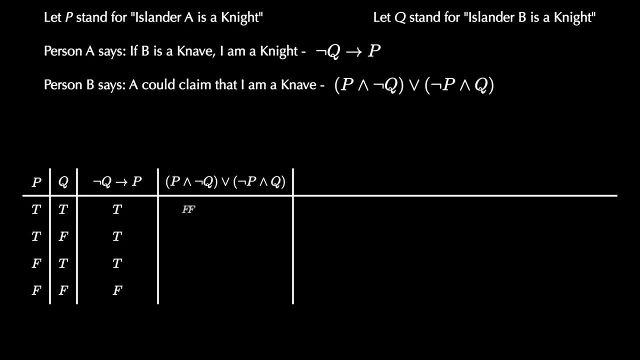 This takes a moment to think about, but basically they have to be of different types. When we go through and we fill in the truth table, we end up with F, T, T, F. like this: We employ the biconditional between the proposition P and the proposition that Person A said. 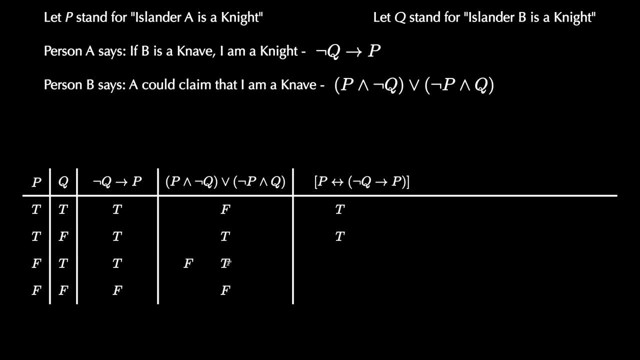 The reason we do this is because knights will tell the truth and knaves will always lie. The biconditional will find if there's a truth teller that's lying or a liar that's telling the truth. Now we do the same thing with Proposition Q and the proposition that Person B said. 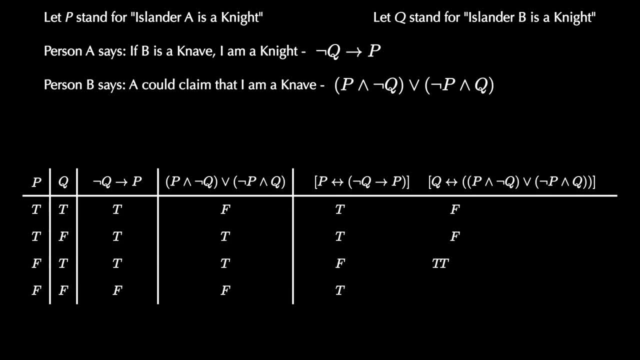 Again, the biconditional will figure out if a truth teller told a lie or if a liar told the truth, Which is not supposed to happen, The biconditional returns a false. in these situations, The two biconditional propositions have already determined when Islander A and Islander B are following the rules of the island. 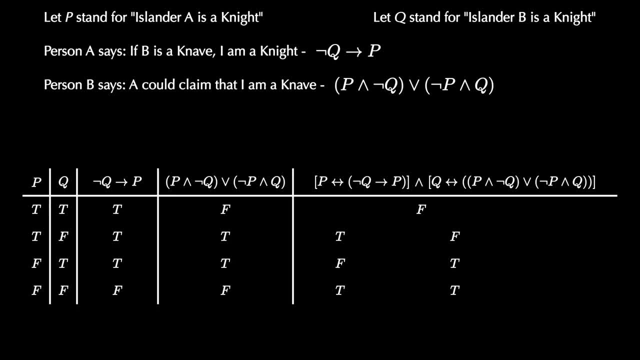 So we AND them together to figure out when both of the islanders are following the rules simultaneously. But now this final column in the truth table has only one true value: in the last row. That means that the last row is the one we must be in, which means both P and Q are false.